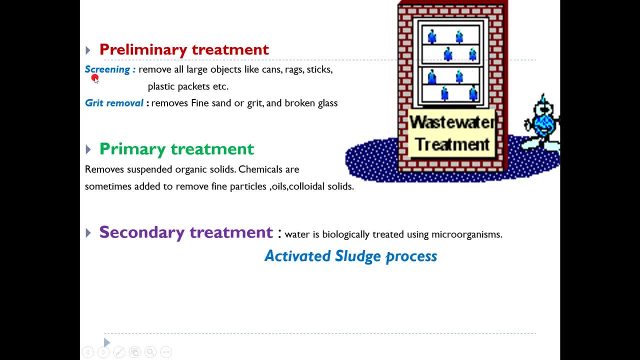 Where we remove the large particles or the objects. So in that we have screening, where large objects like cans, rakes, sticks, everything is removed. Plastic, everything is removed. Grit removes small particles like sand, broken grass. All these fine particles are removed by in the next step of grit removal. Then we have primary treatment, secondary treatment, tertiary treatment. So in primary treatment we remove the. 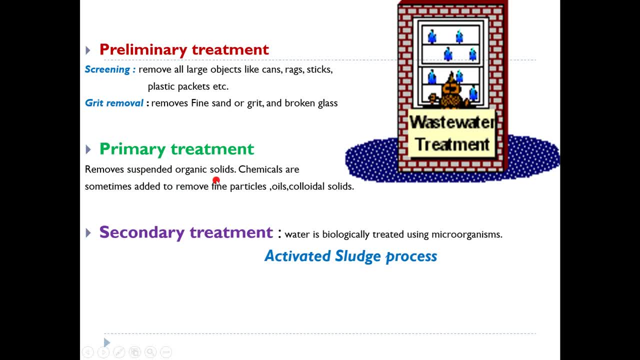 suspended chemicals or suspended solids. So chemicals are added to remove the fine particles. They could be oils, They could be certain precipitates, salts, which are removed by primary treatment, by adding chemicals, carrying out coagulation and everything. And then you have the secondary treatment, where we have the activated sludge process. In this process the water is treated with the microorganisms. 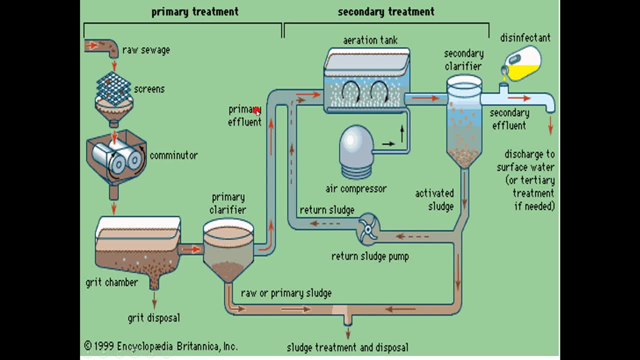 So we are going to study this in detail. So this is how the whole treatment process looks like. This is the sewage water screening grit removal. Okay, this is the grit chamber. Then first we have the primary treatment. All the chemicals, all the solid particles, suspended particles, are removed at this stage and all these suspended particles are removed separately. Clear water is passed through the aeration tank and then through the secondary clarifier. This is your activated sludge process in all. 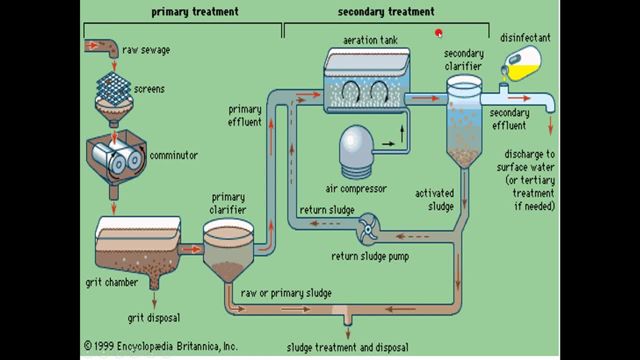 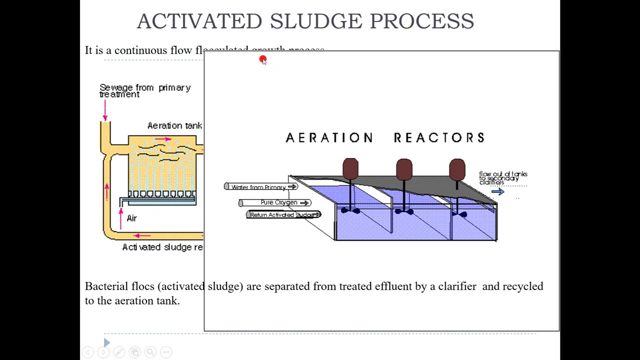 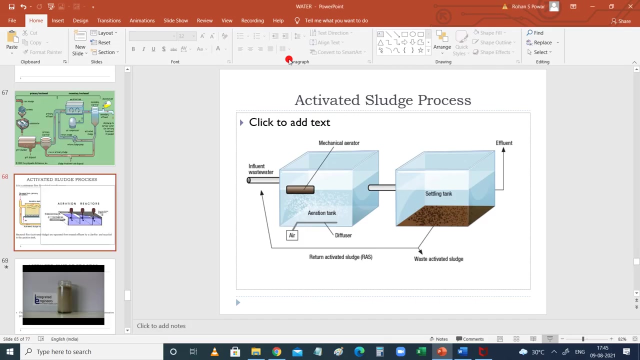 Right, So this aeration and the secondary clarifier this is together makes your activated sludge process And after that, once the water treated obtained from the activated sludge process, it is processed further for disinfection. Okay, So what exactly happens in activated sludge process? It is a continuous flocculate, continuous flow, flocculated growth process. Sorry, I'll just bring it down. 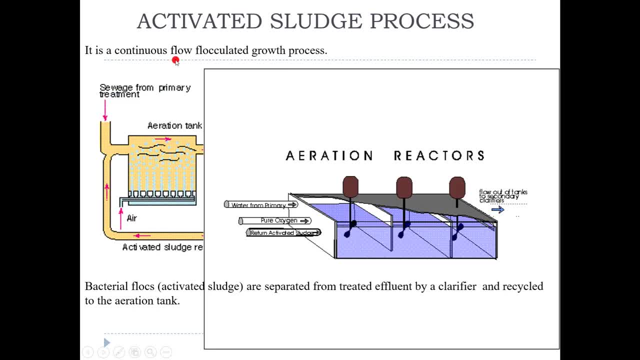 Okay, So continuous flow, flocculated growth process, And in this process, what we have is a aeration tank, So water from the primary treatment is collected in the aeration tank and you have this air which is continuously mixed with this aeration tank, and there are agitators, And these are the bacterial flocks are added in the aeration tank. So bacterial flocks, that is the activated sludge. So this is where the bacteria is growing. 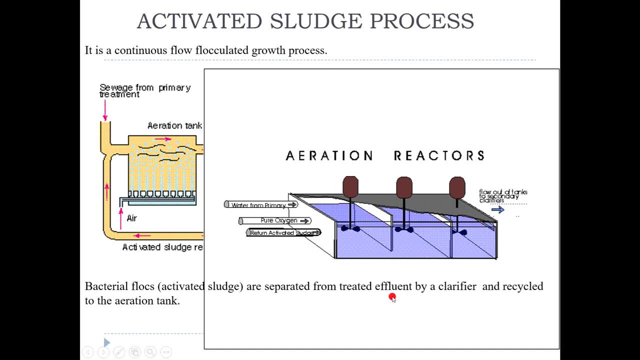 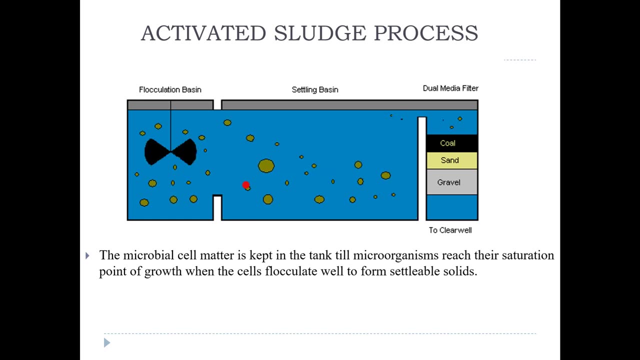 And here the bacterial flocks are separated from treated effluent by a clarifier and recycled into the aeration tank. Here is where your process is taking place. And after that, whatever, because of the bacteria, you know, they start to react with the organic matter or whatever waste that is present in the, in the water And this microbial cell. 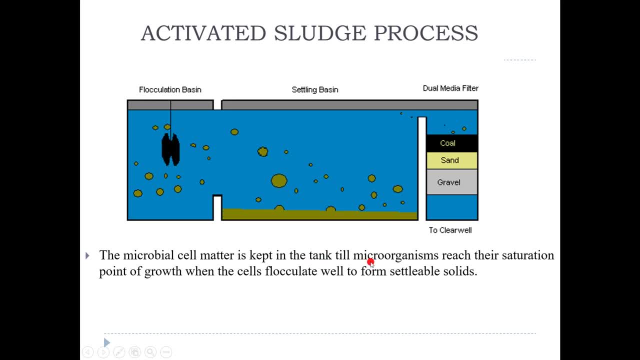 Matter, which is с in the tank. the microorganisms start to grow on that particular matter and they reach their saturation level, and this is when the cells flocculate and form settleable solids. so the whole product starts to grow. they grow in size and then the colloidal particles when they grow. 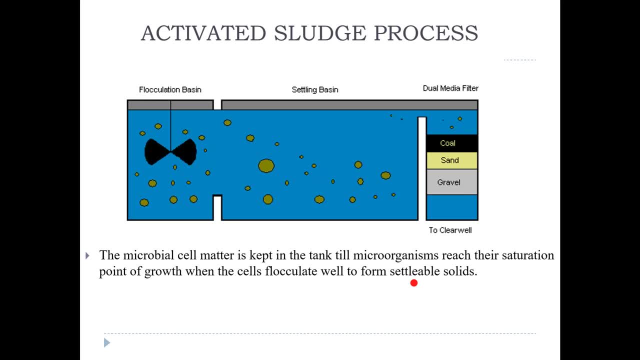 in enough size, their weight increases and then they start to settle down. it's a kind of a coagulation because of the microbial treatment. the bacteria here are responsible to convert the waste into settleable solids, and on the same solids the microbial growth is also taking place. 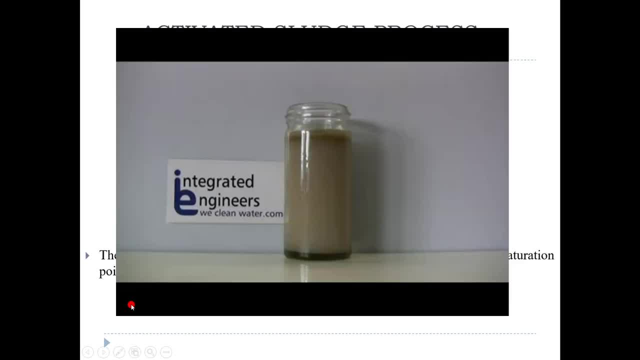 so i will just show you- sorry, there is a small video on this, so you will just understand what exactly i'm talking about. so this is the sludge. imagine this is the water from the primary treatment and you are adding a sort of- you know- bacterial flocks over there and because of this air and the bacterial treatment- whatever, 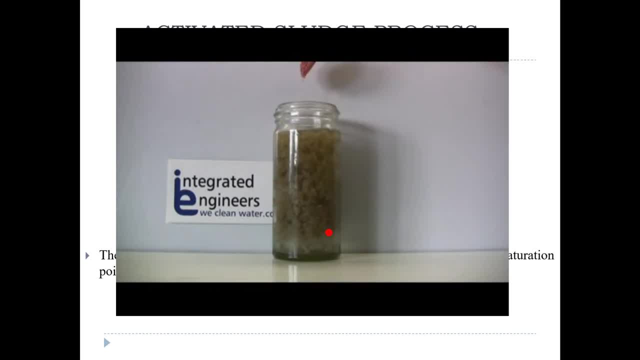 waste is present in the water, it starts to coagulate. you know this is how the dispersed or the diffused solids, coagulate products, are formed, and this is how the sludge is formed. so, on a larger scale, you can consider this as the sludge and see how clear the water has become. 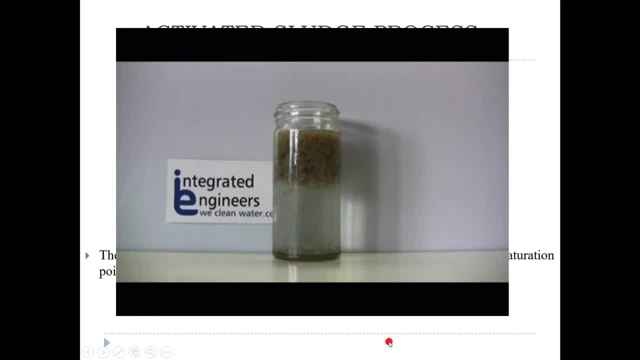 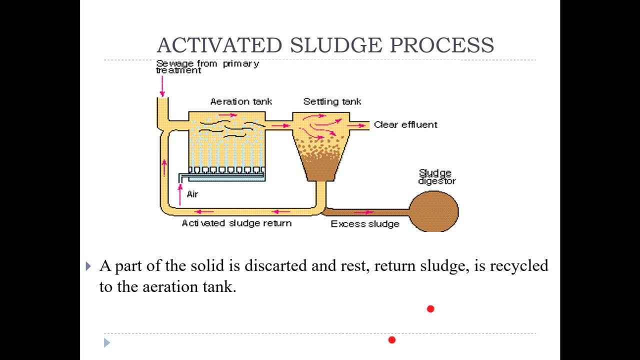 got it. so this is what takes place in the activated sludge process. this is on a small scale. on a larger scale, you get this type of sludge and now, once you get that sludge, we pass the whole thing into a settling tank and the sludge is allowed to settle down. so the part of the solid 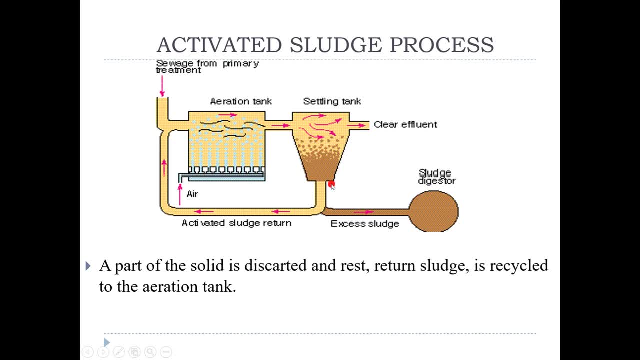 is discarded, this settleable solid which is coming down and settling down, it is now collected in a sludge disaster, and sludge which is rich in bacteria now in some part of that is again- you know- recycled into the aeration tank. so the sludge has more bacteria. same thing goes back into the aeration tank, same. 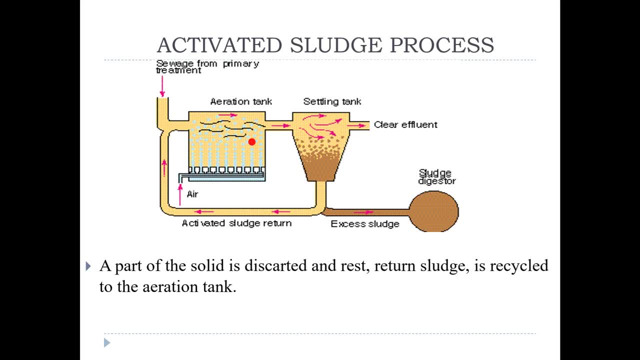 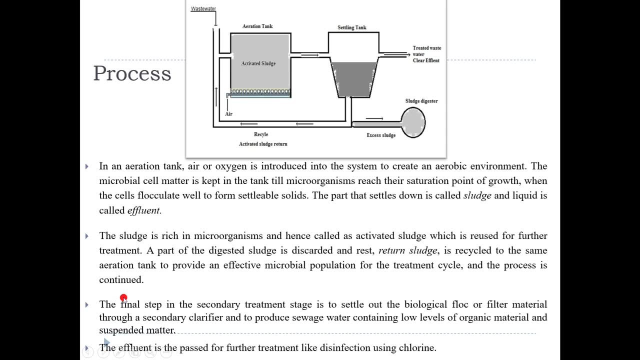 reaction takes place. so this, that is why it is called as a continuous flocculation process. okay, now this is a. this is like if you people are making notes and you have these, you know question answer sort of format, where you have to write a particular question and then you 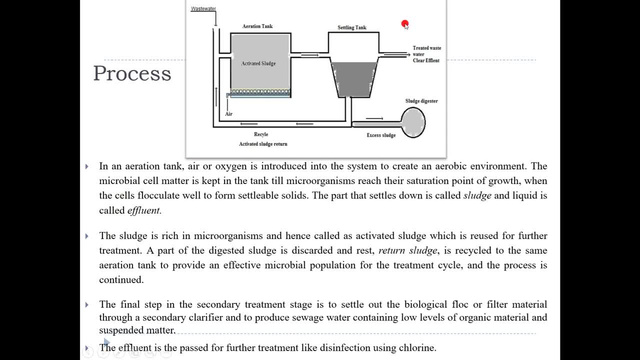 can write a particular answer for the process. you can note down these points and this is the diagram that you can draw, and it's the same thing. like you have the aeration tank in which the oxygen is mixed with the water from the primary process, sludge is formed, settleable flow solids are formed. 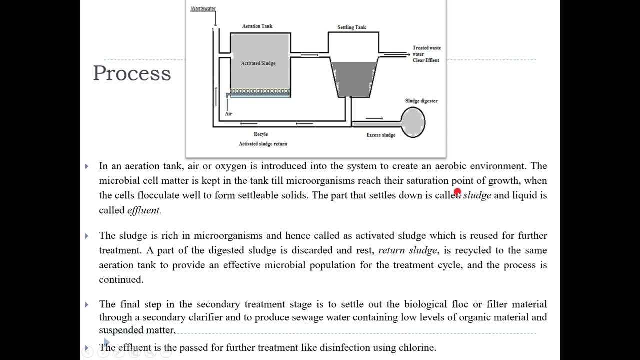 they settle down and part of the sludge settles down. that is called sludge the liquid, the clear, so liquid which is formed. it is removed from the top and the sludge is written back into the aeration tank tank and whatever water is obtained from this process is passed into further. 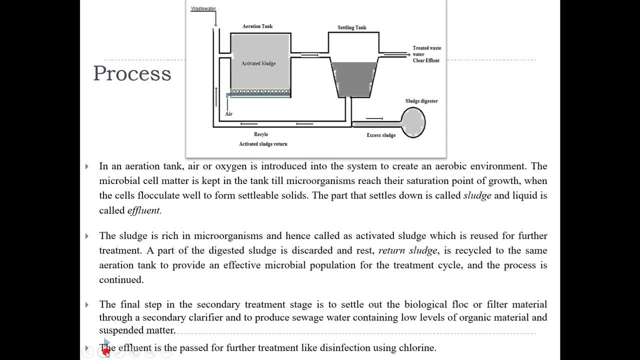 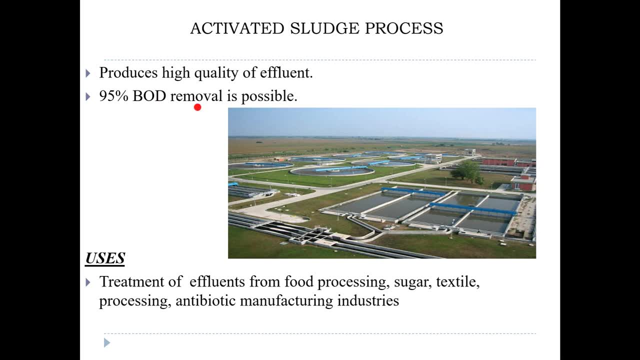 treatment for, like disinfection with chlorine. okay, so this was all about activated sludge process. the process is very good to clear, purify water on a large scale. so most of the wastewater treatment plants have this activated sludge process. it produces a very high quality of affluent. you have seen how. 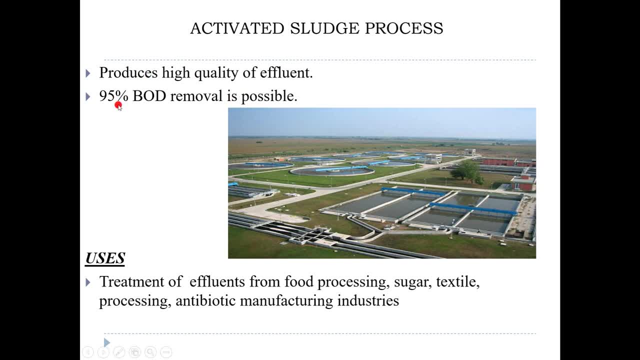 the quality of the water changes. from that small video that I showed you, 95% BOD removal is possible, so most of the organic matter is removed from that. okay, BOD is biological oxygen demand. I made a separate video on BOD and COD. you can. 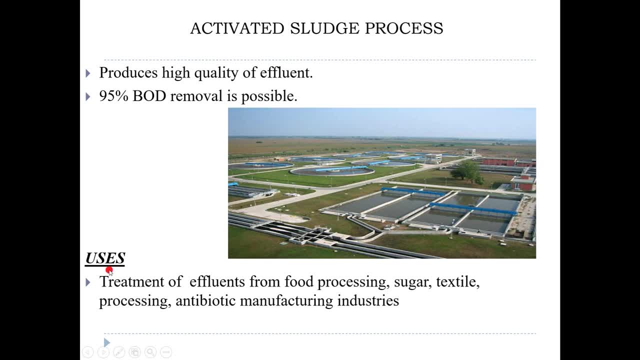 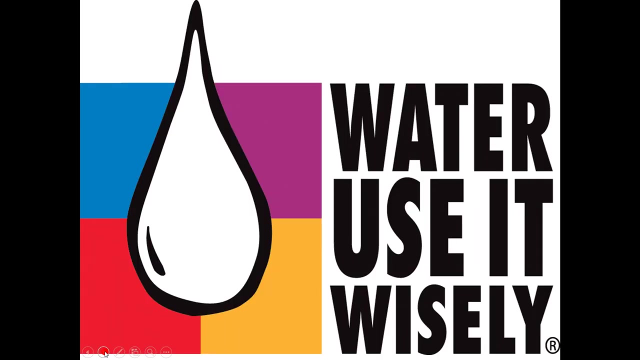 watch that and what is the use use of is very, very efficient. it is used for treatment of effluents from food processing, sugar, textile processing, antibiotic manufacturing industry. very well in large-scale industries. wherever wastewater is generated, you can use this process for purifying the or cleaning up the waste from the water. 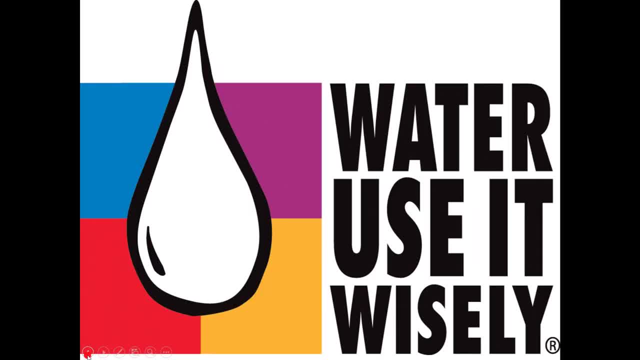 okay, so that was about activated sludge process. do watch the other videos on the water chapter. thank you.